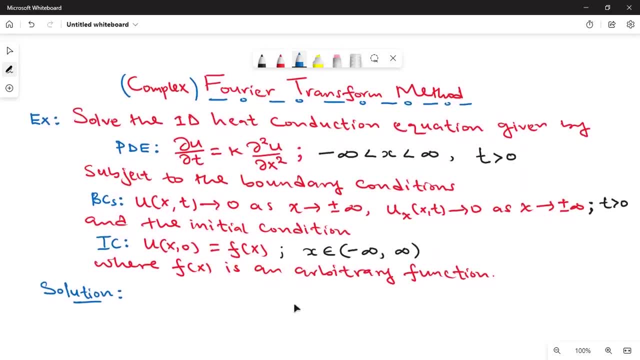 So how do we go about this problem? Using what we call the complex Fourier transform method. Remember, we have three types of Fourier transform: The complex one, which applies for the complete domain from negative infinity to the positive infinity. I will also look at the Fourier cosine transform and the Fourier sine transform. 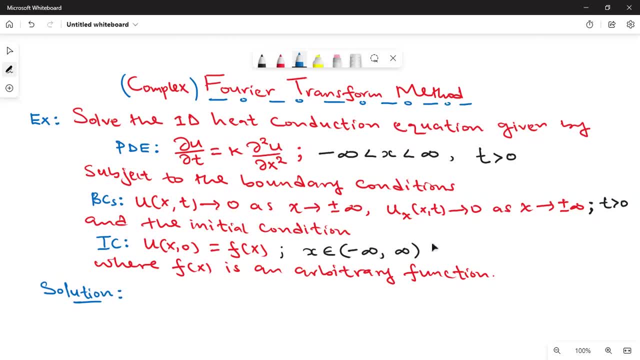 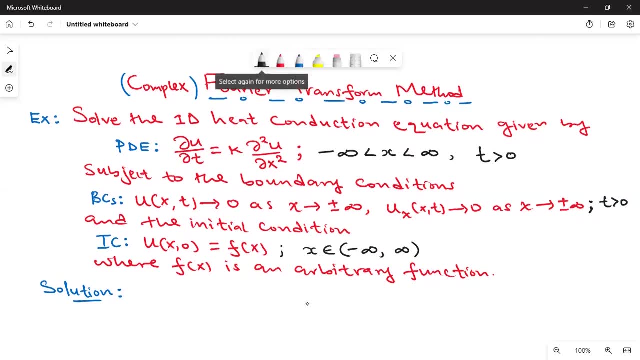 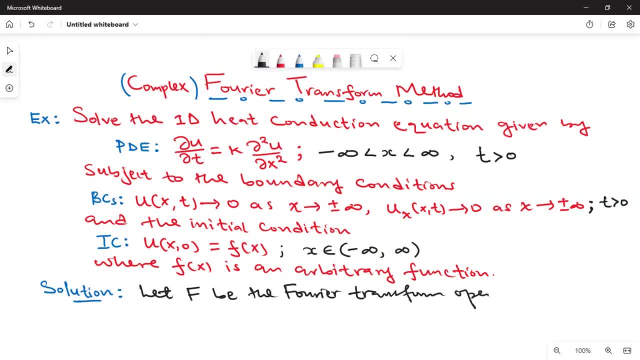 Let f be the Fourier transform operator. Let f be the Fourier transform operator. So we will operate with the f. Look at our PDE. The k in the PDE is thermal diffusivity, Thermal diffusivity. Now what you do is to operate with f on both sides of the given equation. 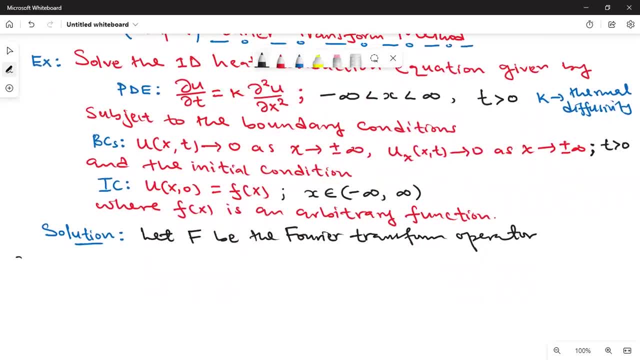 So the first step, Write step one. We are going to operate with f on both sides of the PDE. So what are we going to get? You write Fourier transform of partial u. You write Fourier transform of partial u. You write Fourier transform of partial u. 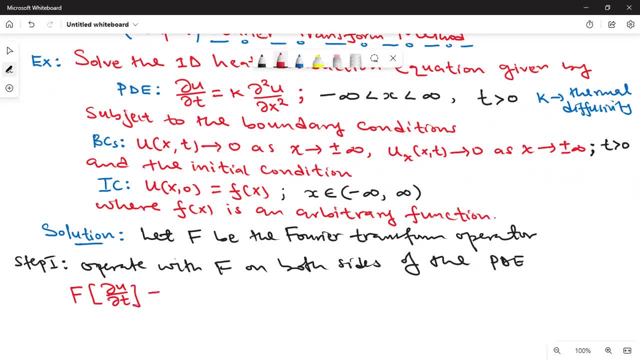 Partial t is equal to Fourier transform of k. k is a constant times second partial derivative of u with respect to x twice. Remember this Fourier transform is in the variable x. So we are saying: let f be the Fourier transform operator in the x variable. 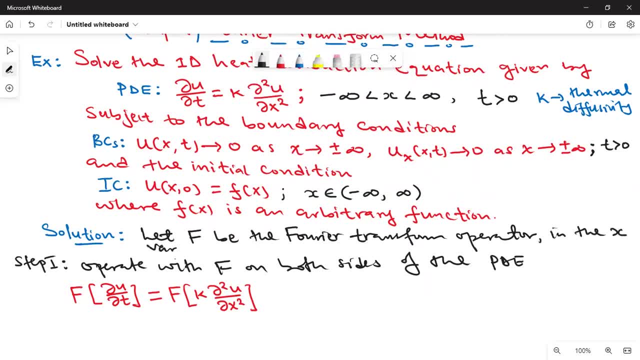 why are we saying in the x variable: Fourier transform is simply: should operate on that variable which extends from negative infinity to positive infinity, the complete interval. so when you have a variable that starts from 0 to positive infinity, you cannot operate on that variable, only operate on variables. 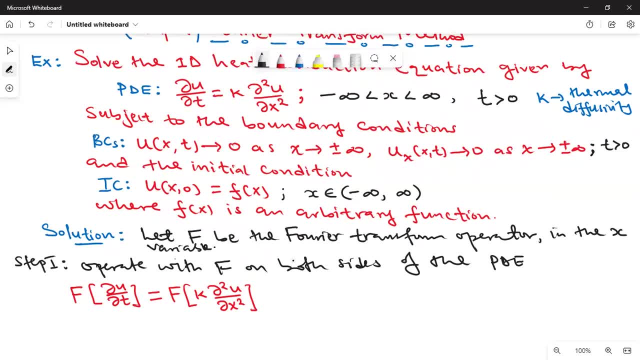 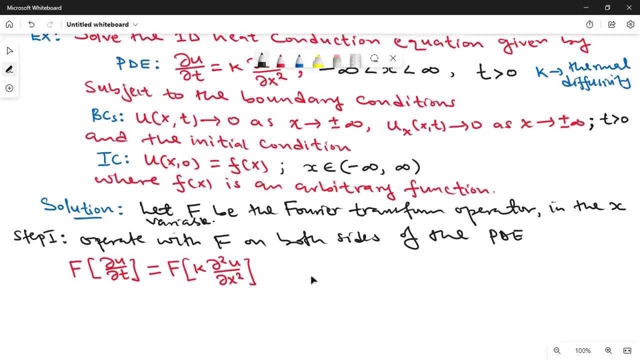 which extend from negative infinity to positive infinity, and so we are going to operate on the variable x. so when you operate on the variable x, you assume that the t variable here is a constant with respect to the operator f. now you see, k is a constant and this can now be factored out. 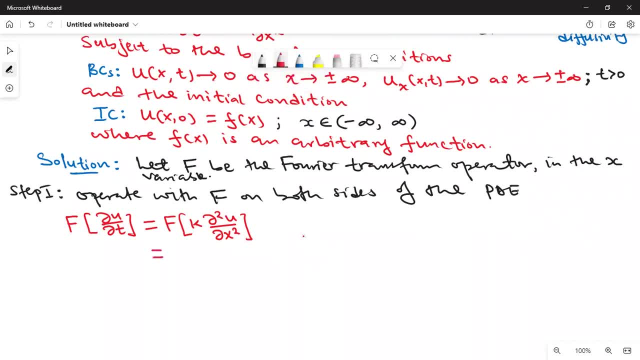 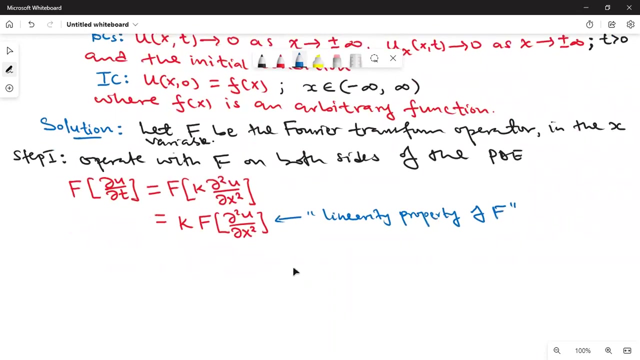 because of the linearity property of f. so k constant. then a Fourier transform of second derivative of u with respect to x, twice. what have I used here is the linearity, linearity property of the operator f. so because we are saying we are treating the variable t as a constant. 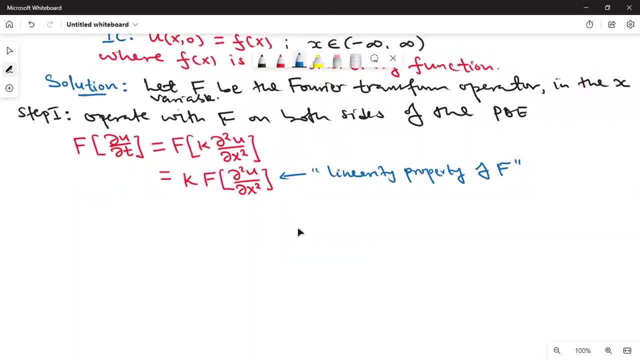 and only operating on the variable x, our transform of the derivative with respect to t will be this one. so it will be now o d e, d, d, f, d, t. I mean d, d, t of the Fourier transform of u. remember u is a function of x, t. 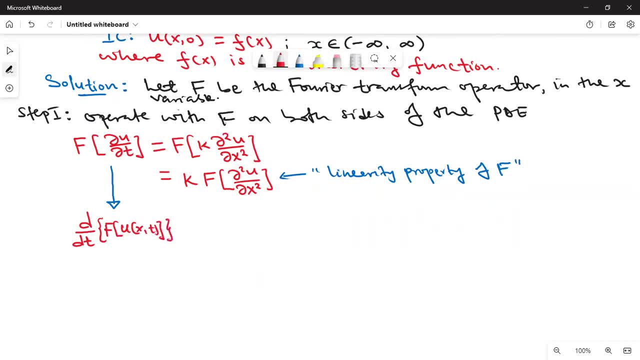 Fourier transform of u of x, t. that's what you get when you transform that derivative is equals to k is a constant. when you transform derivative with respect to x, you need to get, of course you know that in general, the Fourier transform of u is a constant. 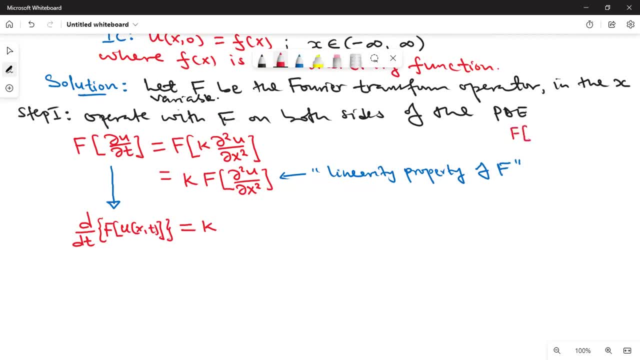 the Fourier transform of the nth derivative of u with respect to x raised to n. this will always give you iota times omega raised to n times the Fourier transform of u. that's what you need to get in general. so when you have second derivative, we will now talk of. 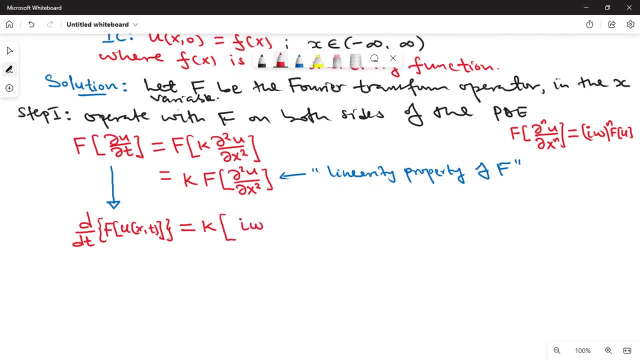 iota times omega raised to two, because our n is two times the Fourier transform of u, of x, t. that's what you get. and remember i, what you are calling iota, is the square root of negative one, so this means that i squared will be equal to negative one. 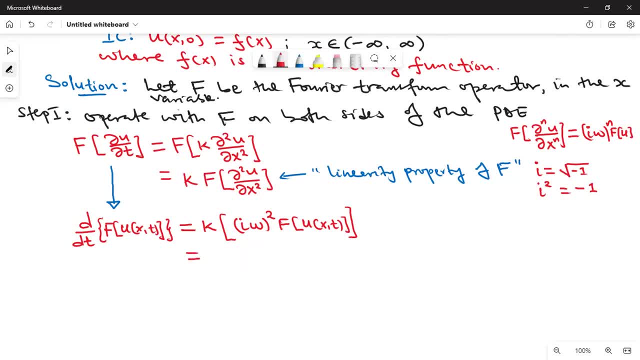 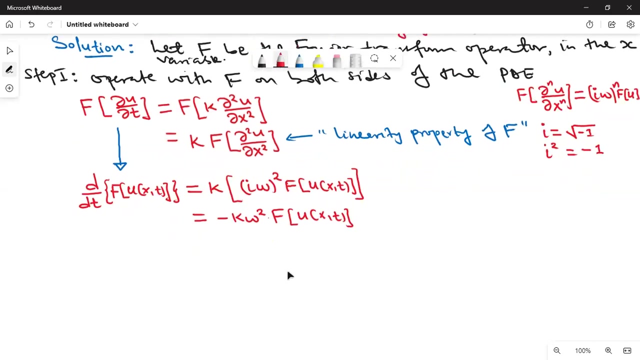 so that on the right hand side we can now get this as negative: k omega squared, y negative because of the i squared, then times the Fourier transform of u of x, t. that's what you have. i can take everything to the left hand side so that i have: 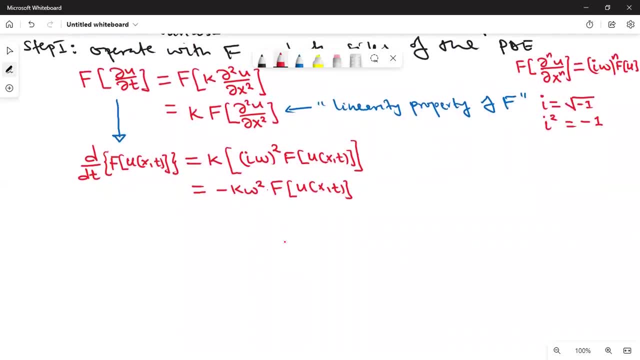 an equation that i can solve easily. so you can write: or d dt of the Fourier transform of u of x t, then plus or minus k omega squared Fourier transform of u of x t. this should be able to give us zero on the right hand side. this one here is an ode. 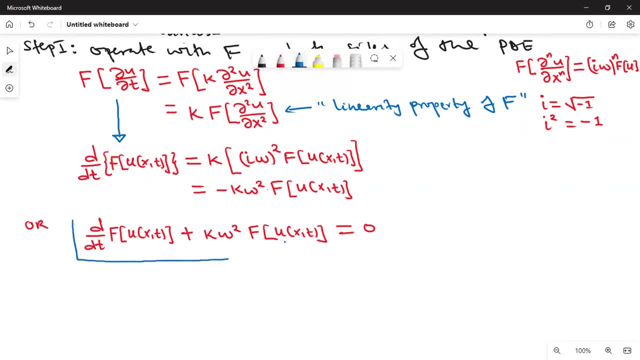 this is an ode of the first order with the constant coefficients. of course it is separable. you could also solve as a linear ode or you can solve this in the d operator. this is a linear ode or simply an ode of first order with the constant coefficients. 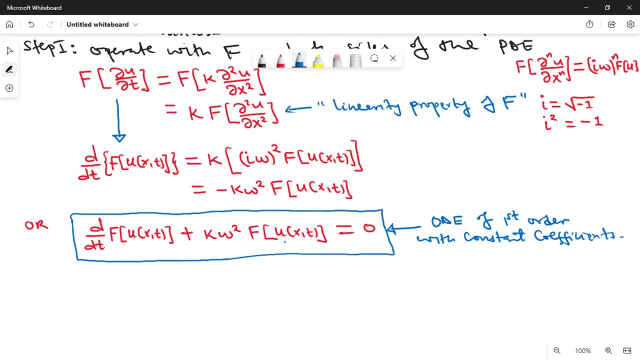 there are three methods of solving it. you could use d operator, you could use the integrating factor method, or you could solve this as a separable or the e. we are still going to get the same answer. so i want to use d operator, so let d capital be. 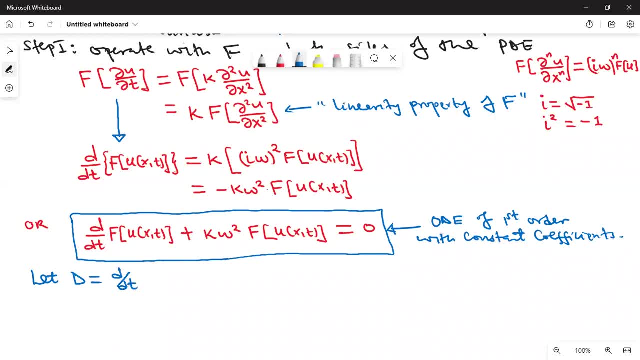 derivative with respect to t. so if that is the case, then our equation will now be: d plus k. omega squared, operating on the Fourier transform of u of x, t should give us zero. of course, you should also take note that it is a homogeneous ode, because the right hand side is zero. 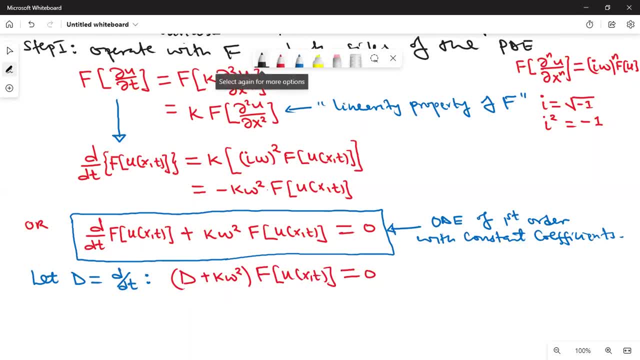 so what is the auxiliary equation? let me talk of aux auxiliary equation. you know you need to create the coefficient of that Fourier transform to zero. so d plus k, omega squared is equals to zero. so what about the roots? it's just one root. when you make this a subject, 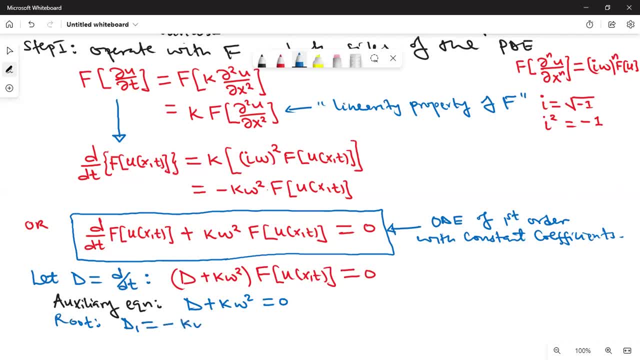 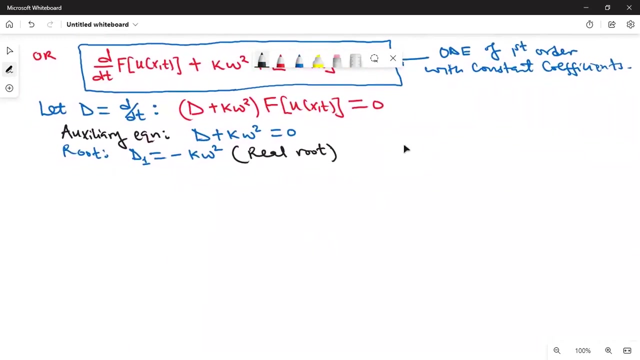 you are going to get negative k, omega squared, and this is a real root. real root: when you have just one real root, how should you write your general solution so you can say that? therefore, therefore, we know that now, the Fourier transform of u, of x, t, should now be equal to a constant. 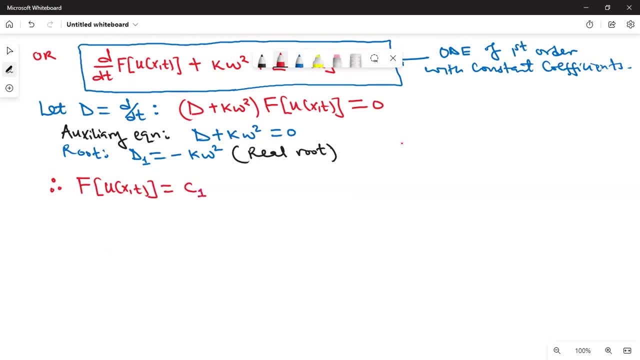 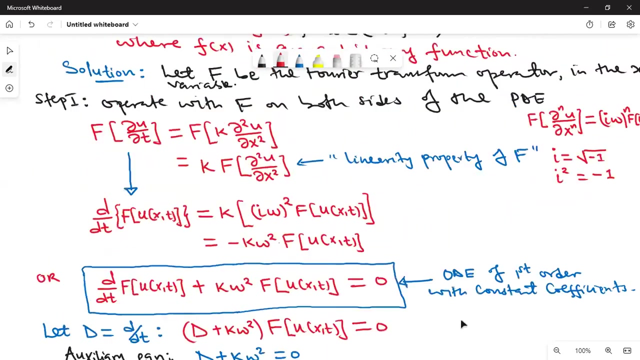 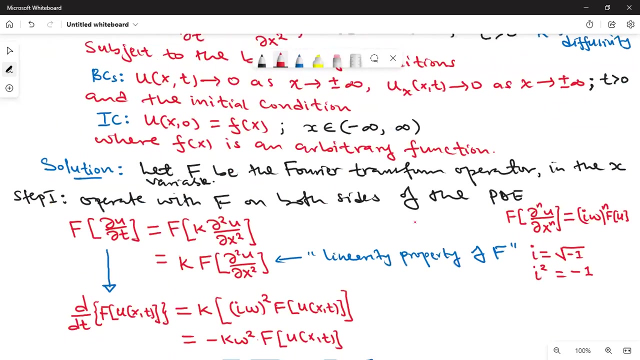 call it c, or even c1, exponential negative k, omega squared t, where c1 is an arbitrary constant which we need to determine, remember. somebody might be asking: what do we do with the boundary condition? those boundary conditions are what gave us this formula. when you apply those boundary conditions, 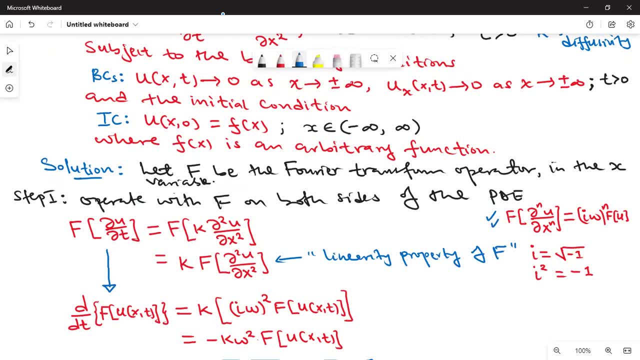 you get this formula that we have used in our equation, so already these boundary conditions have been taken care of. what you need to apply is the is the initial condition. so I did. you don't need to derive this, because already this was derived in the previous lecture. 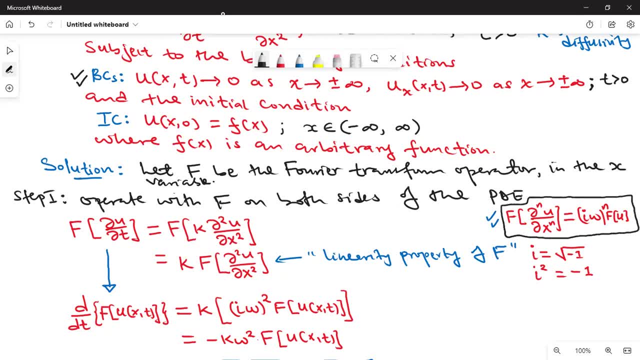 so you only need to apply this formula and to get this formula, it is derived from the boundary conditions. I hope that is. that point is taken. so now we need to apply the initial condition so that you see whether we are going to get the arbitrary constant c1. 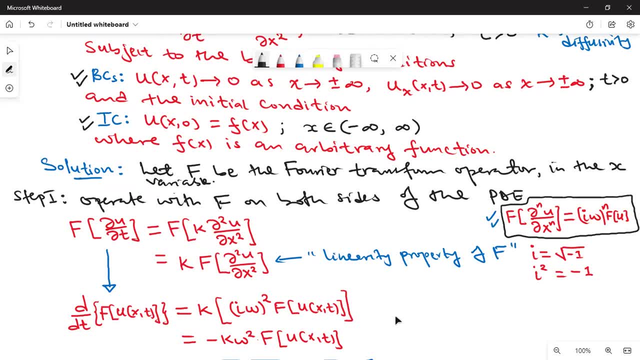 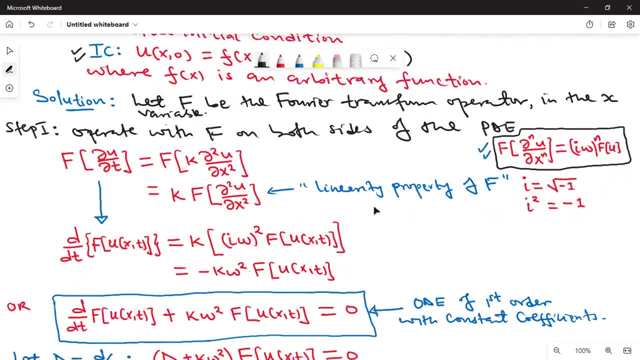 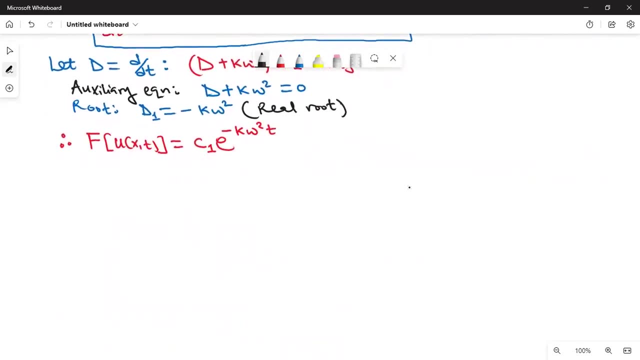 so that will be step two. step one: we have solved it and now we have our solution in terms of the transform. so step two, step two: you write: apply the initial condition. what are we told? that u of x0 is equals to a function of x. that's an arbitrary function. 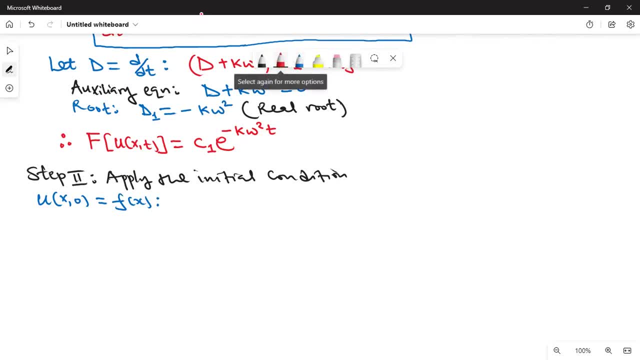 so you also need to take the transform on both sides. so therefore this means that the Fourier transform of of u of x0 shall be equal to the Fourier transform of f of x. let's call this u capital, a function of omega. so that means in this equation: 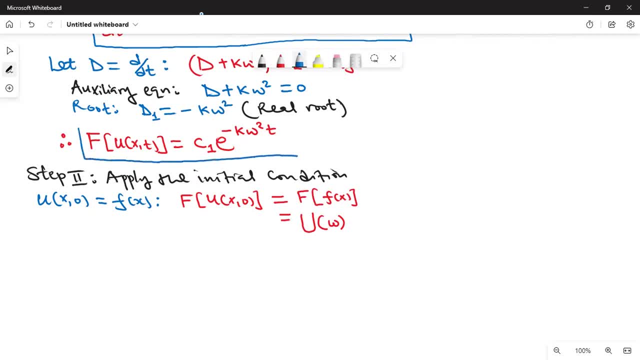 this solution that we have found, I need to substitute t is equals to zero, so that our transform will be equal to u of omega. so when I put put, t is equals to zero and the Fourier transform be equal to u of omega in this equation, the one that I have ticked, 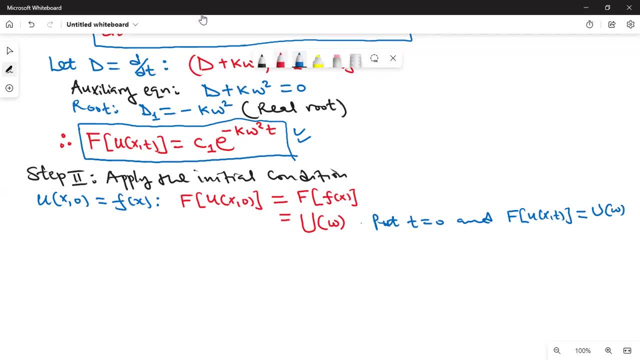 so what are we going to get? it will be: u of omega is equals to c1 times exponential. because time is zero, this will be exponential zero. so this simply means that your c1 is equals to u capital of omega. so therefore, if you replace it back to that, 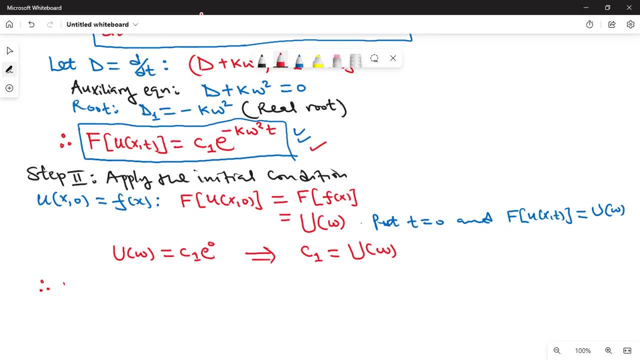 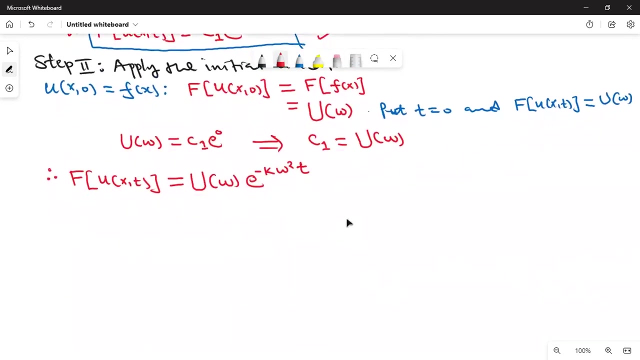 solution, this one, we get Fourier transform of u of x, t is equals to the capital u of omega times exponential negative k, omega squared t. that's the second step. we have applied the initial condition to get that. then the next thing, of course. let me bracket this one. 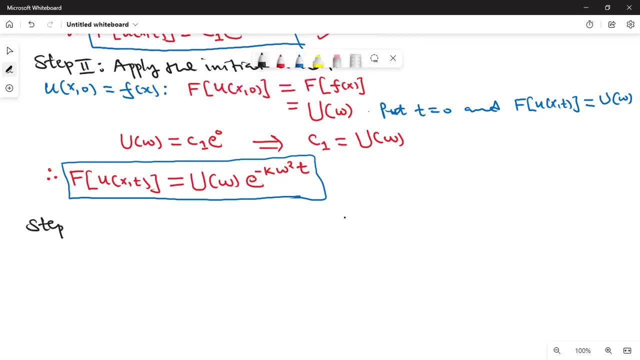 the last step, step three: you now operate with, with f inverse, that is, the inverse Fourier transform on both sides, on both sides of this equation, the one I have ticked now, when you operate with f inverse on the left hand side, you are going to get u. 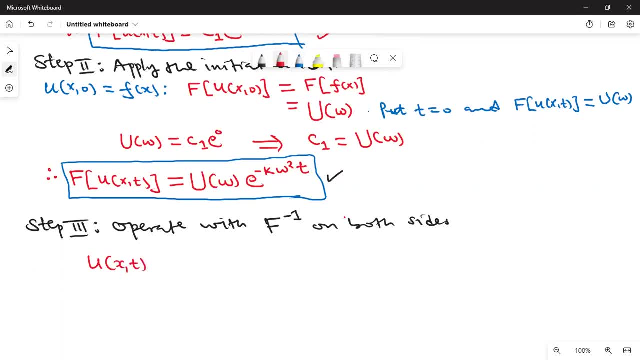 of x t. remember f and f inverse are inverses of each other. so f inverse of f is an identity operator. so we remain with the u of x. t is equals to f inverse of u. capital, a function of omega times, exponential negative k, omega squared t. 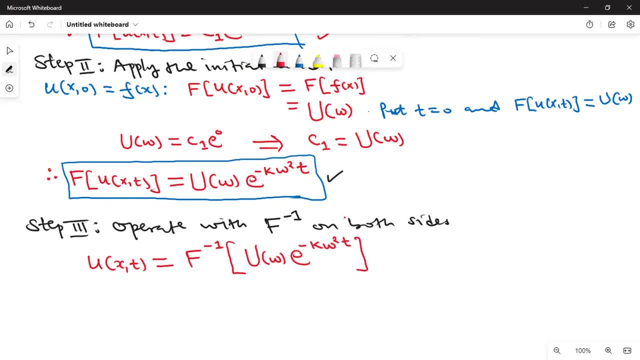 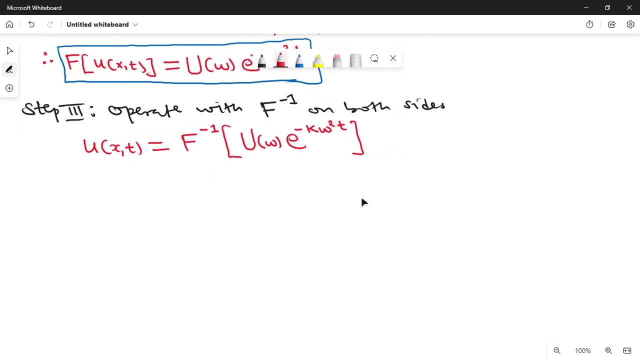 now the task is: how do you find the inverse transform of that function? that is the question. so this is look at our definition of the inverse Fourier transform. I am going to use convolution theorem. why? because these two are- these are- function of omega. again, this one is a function of omega. 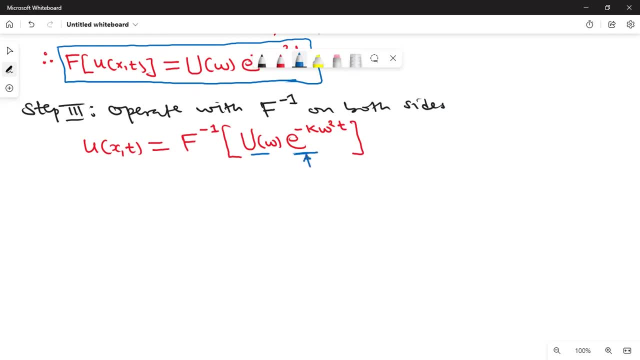 let this one, let this one be g, a function of omega and t. so, because we have a product of two functions of omega, we use convolution theorem. so, use convolution theorem, since we have a product of two functions of omega. that is when you are getting the inverse transform. 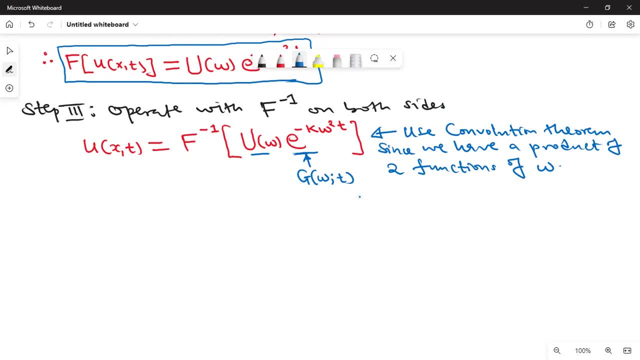 so you remember the convolution theorem, remember the convolution theorem. let me state it: convolution theorem that I can use another color, that f inverse of, let's talk of. let me look for a better function to use: f inverse of: u of omega times, g of omega t is the same as. 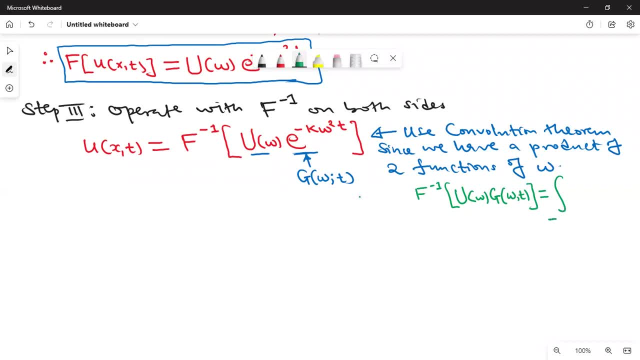 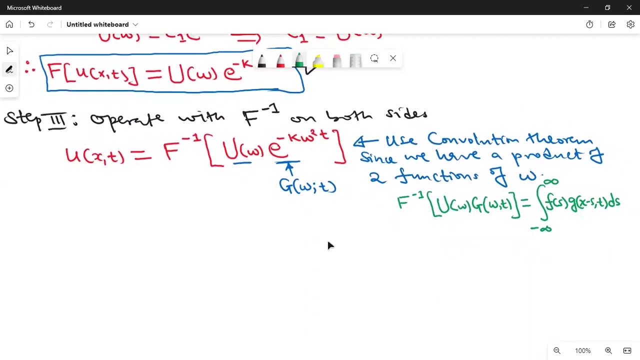 the integral from negative infinity to positive infinity of f of s, times g of x minus s, t, ds. that is the convolution theorem. convolution theorem. now it is f, f of s and what is g. you can say where f of x is the inverse, f inverse of u. 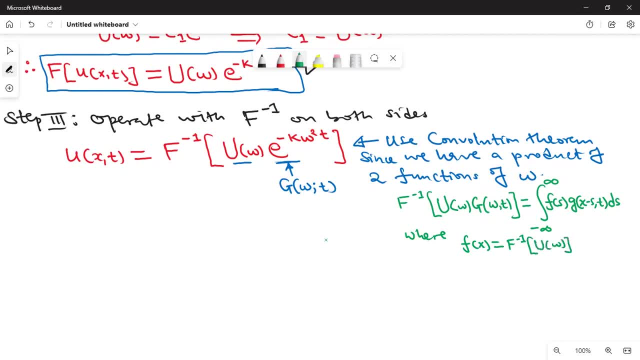 of omega and g of x. t is f inverse of g of omega t. so if you know f and g- the small one- then it is easy to get the inverse of a product of two functions of omega. this is called convolution theorem, so I can. this is a special. 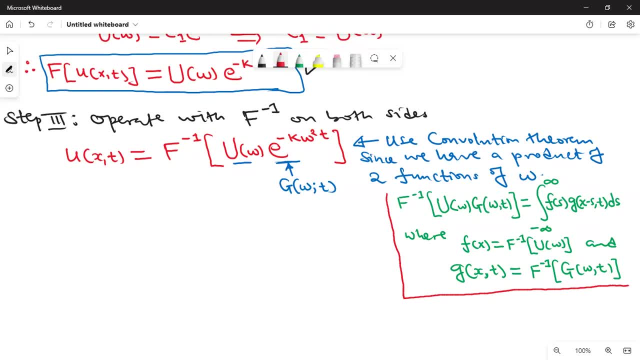 theorem that you are going to use. let me bracket it that way. so, therefore, we expect that this can now be written as the integral from negative infinity to positive infinity, of f, of s times, g of x minus s, t, ds. so what do we need to find already? 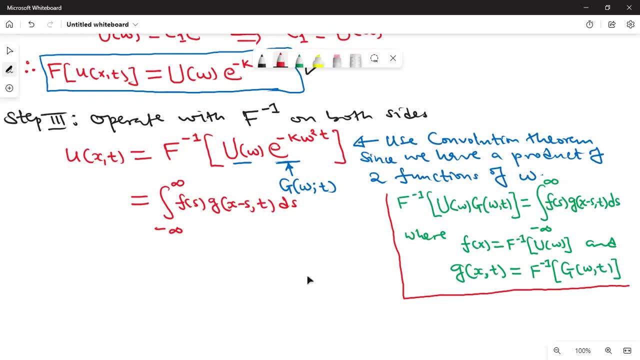 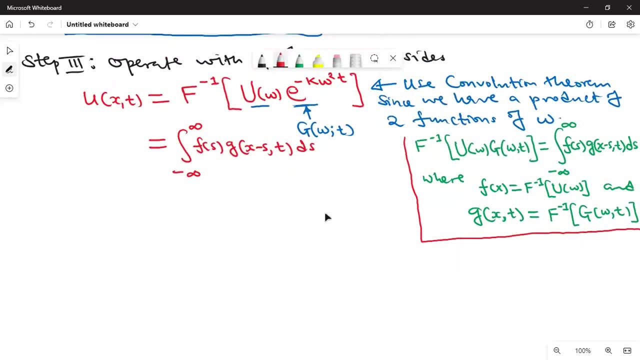 we know we don't know f of x. it was an arbitrary. so we only need to know where to find g of x t, because once you know it, it is easy to find g of x minus s times t. so I'll call this equation star. I'll call this equation star. 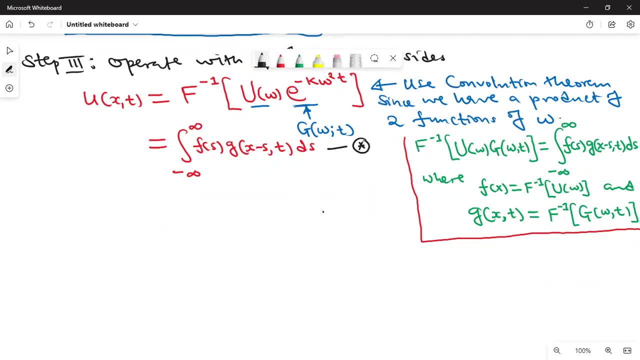 now let's find the function, the small g, as a function of x and t. of course we know that f you can just write where- let me use another color- where f of x is equal to f, inverse of u, of omega, and g of x, t is equal to. 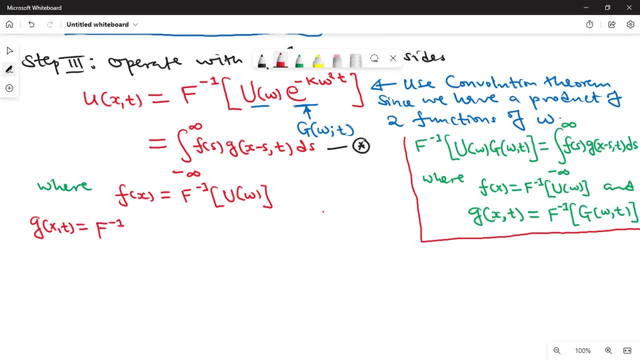 f inverse of the other function. look at this one exponential negative k omega squared t. another thing you need to take note of. also take note another color, that when we talk of f of x, we know that f of x is equal to f of x and t. 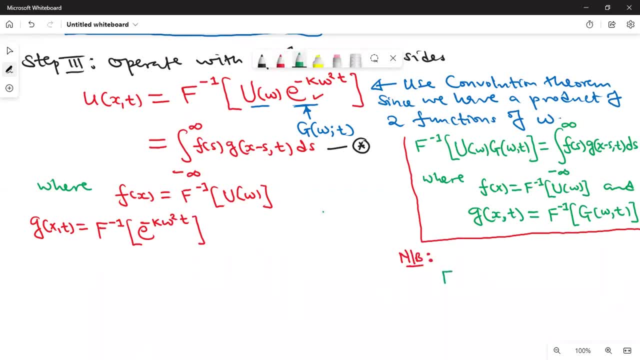 but when we talk of the inverse, Fourier transform, f inverse of a function of omega, let's say f inverse of g of omega t is defined by one over two pi and times the integral from negative infinity to positive infinity of that function, g of omega t times. 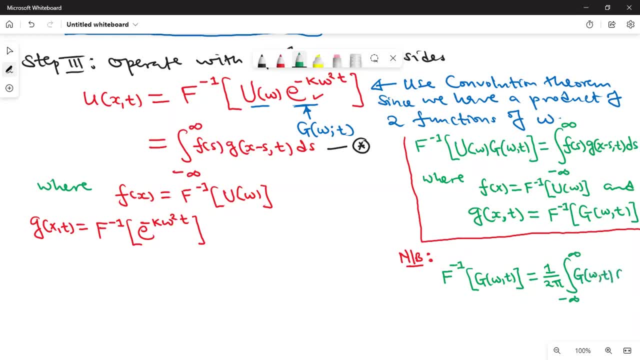 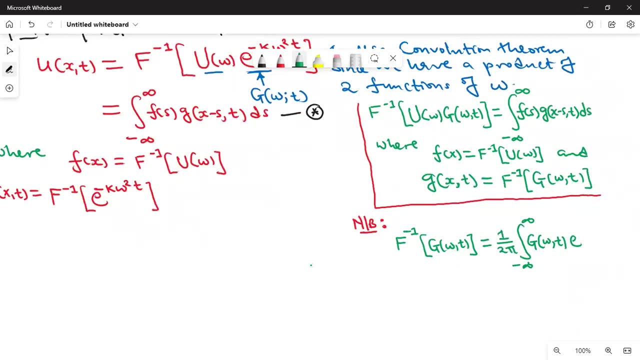 exponential. let me take this to the left so that i can write here: exponential i, omega, x, d, omega. that is how to find the inverse transform, the inverse Fourier transform of any given function of omega. this formula is very important, very, very important. this is what we are. 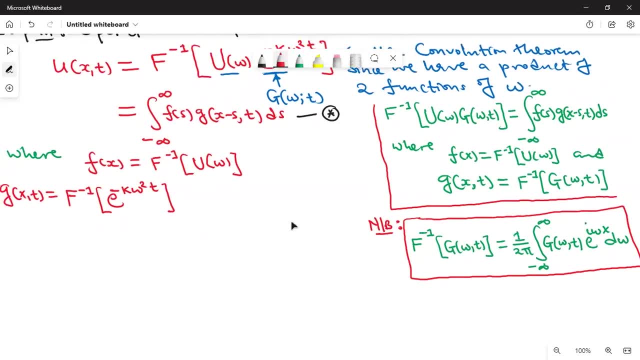 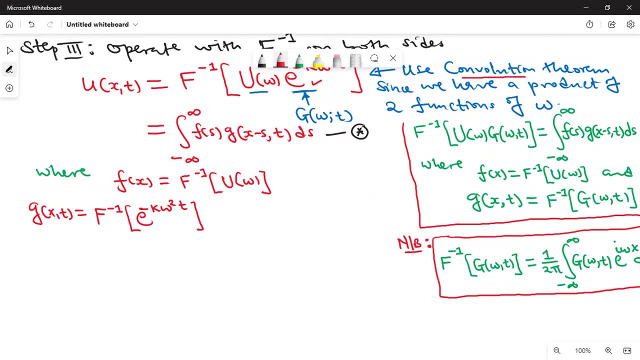 going to talk about in the next lecture. we will talk about how to find the inverse transform. so how will this look like? it is now equal to infinity of exponential negative k, omega squared t times exponential i, omega x. this is the omega and this you can, as. 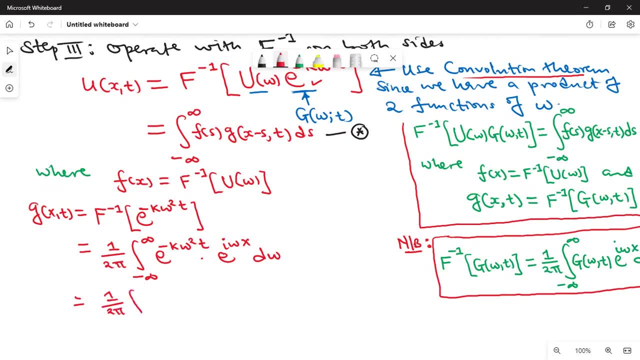 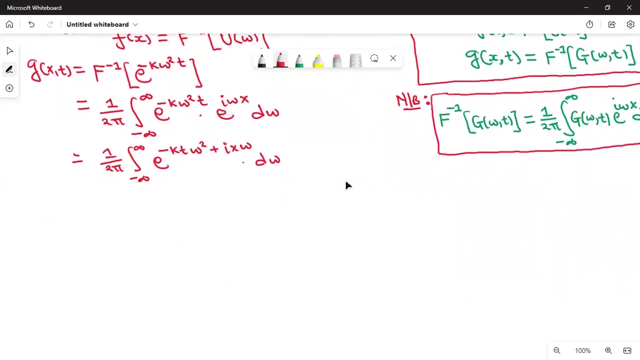 well, write as the integral, from negative infinity to positive infinity, of exponential negative kt, omega squared plus i, x, omega, d, omega. now how do you integrate it? that's the question- is a quadratic expression, our exponent, this one here, is quadratic, this one is quadratic, so what do? 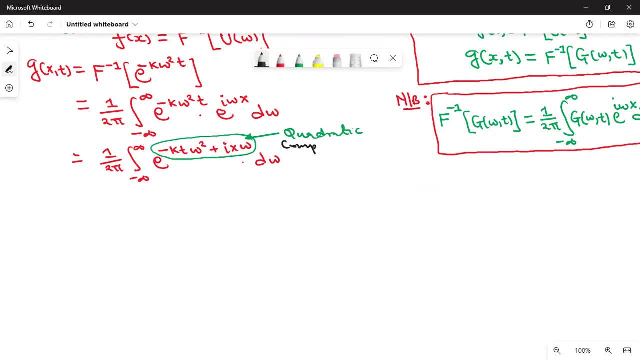 we use use complete, you complete the square, complete the square in that exponent because it is quadratic. so let me complete the square. this side. remember that negative kt omega squared plus i x omega can be written as negative kt bracket omega squared minus i x over kt times. 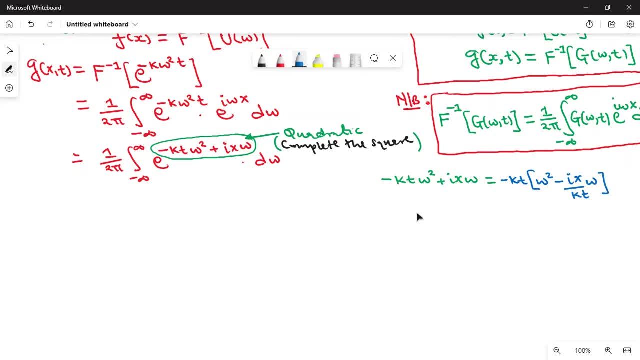 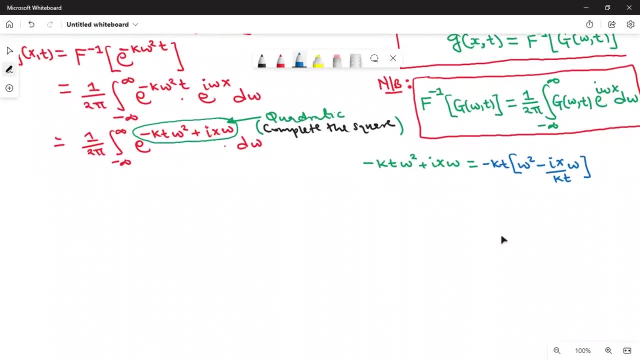 omega. i have factored out the negative kt. why? because you see when you are writing the equation you are going to write negative kt omega squared minus i x over kt omega. i need to add a number c plus a number c. how do we get the number? 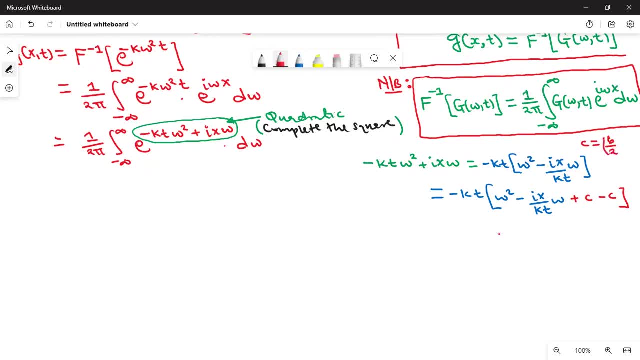 c. it is always equals to b over 2 squared. b over 2 squared. what is our b? our b is the coefficient of omega, so this is our b and this is our b. so this is our b over 2 squared. so what is our b? 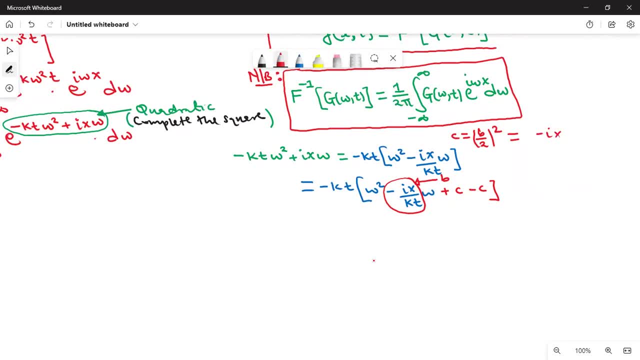 over 2 squared is negative. i x over 2 kt, and which is the same as negative, i squared x. squared over 4 k. squared t squared. that's what we have and which you can simplify to get remember: i squared is negative, i squared minus i. 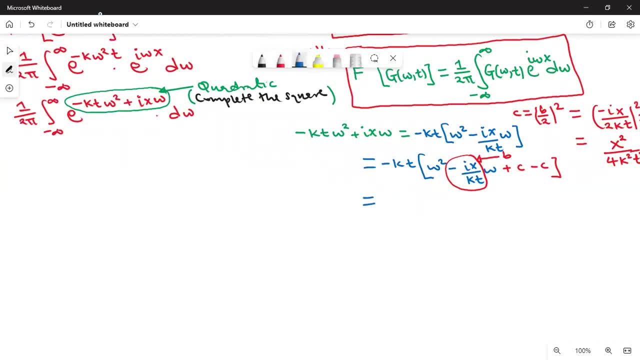 x over k t omega. so we are adding x squared over 4. i x over k, t omega. so we are adding x squared over 4, k squared, t squared. that's the c that you're adding. we also subtract the same c, x squared over 4. 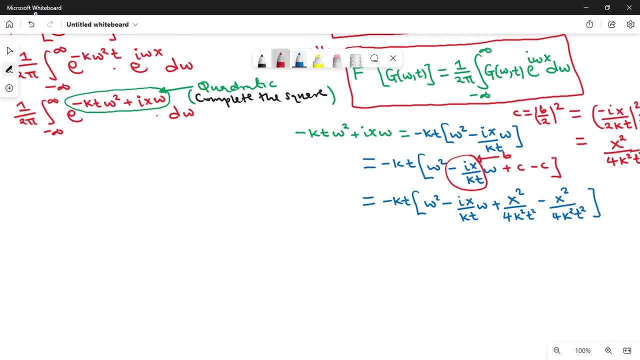 k squared, t squared. you subtract and you also add the same. that is now a perfect square. so that will give us negative k t. when you factorize the first bracket, you're going to get omega minus i x, omega minus i x over 2 over 4. 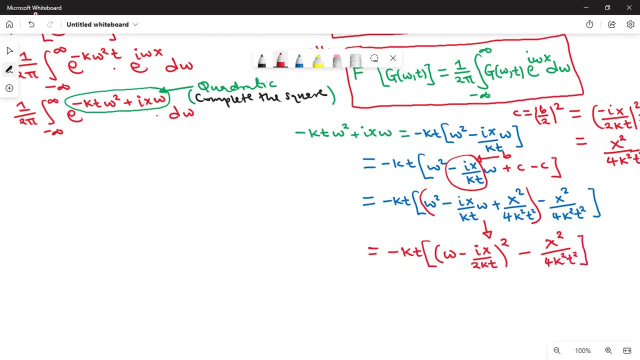 k squared, t squared. that's what we get if I take, if I take this one inside the all of this negative k t, how can it be written over? x over 2 k t? this is supposed to be squared then, plus k t, x squared over 4. 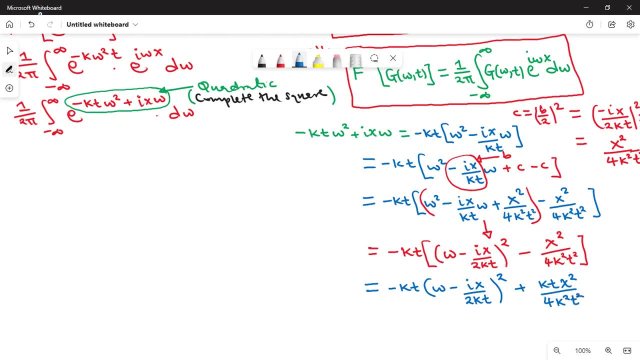 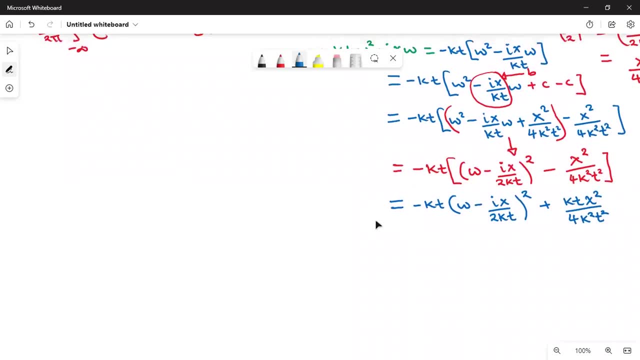 k squared, t squared, and now you can simplify. you can. now we are going to get: this is equals to negative. remember: k t is the same as the square root of k t and this is, squared, is the same thing. times omega minus i x over 2. 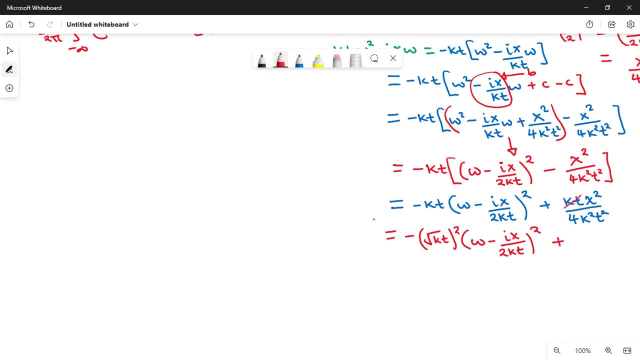 plus. you see, the k t will cancel with these powers, so that we have x squared over 4 k t. that's what we have so now. you can now take this: the root k t plus the square root of k t times, omega minus i x times. 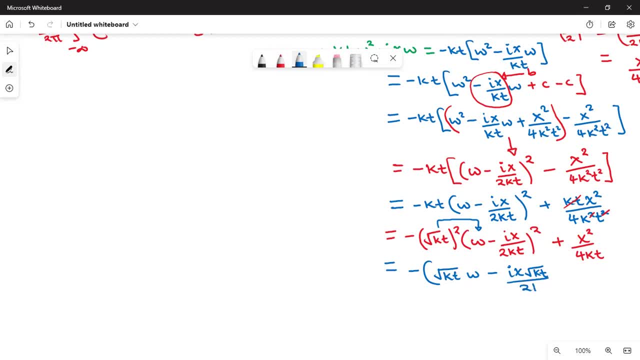 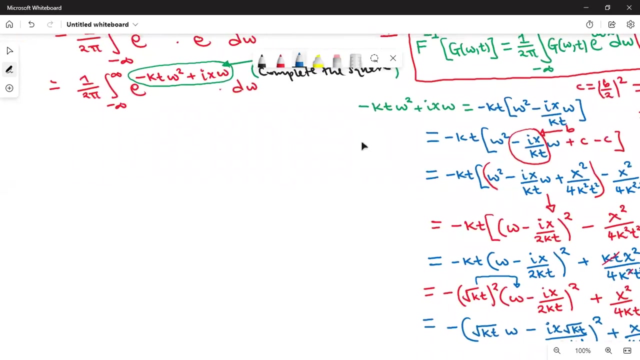 root k t over 2 k t. this is squared plus x, squared over 4 k. so when we complete the square we get that. then now we go back here and replace it, so that in our integral we are going to write this: it is now equal. 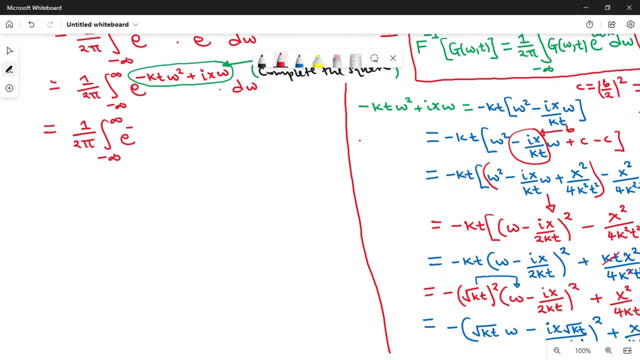 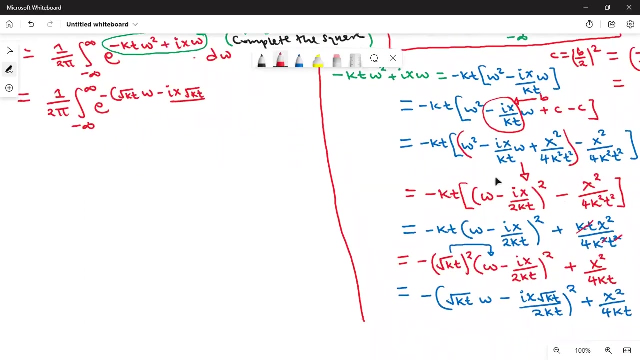 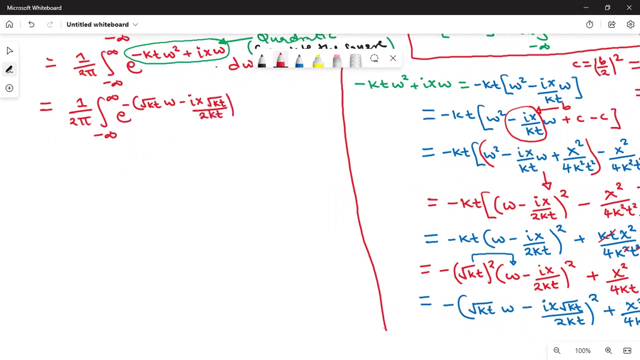 to What did we find? We got negative. the square root of kT, omega minus iota x. root kT over that was- let me check- 2kT over 2kT. This is squared. then I can see this plus x squared over 4kT and it is supposed to be integrating with respect to omega. 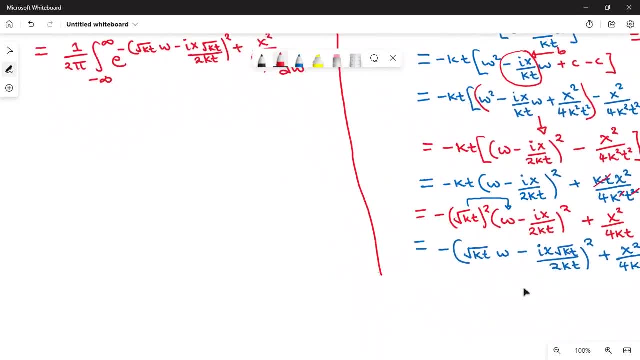 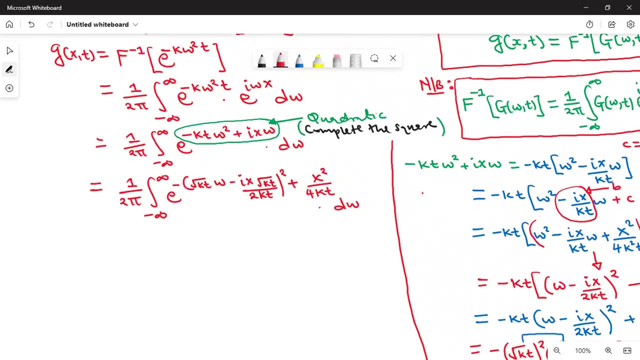 That's what we got when we complete the square, So how else can you write this? This can as well be written as: 1.. 1 over 2 pi. the integral of negative from negative infinity to positive infinity. exponential negative. the square root of kT times omega minus iota, x times root, kT over 2kT. 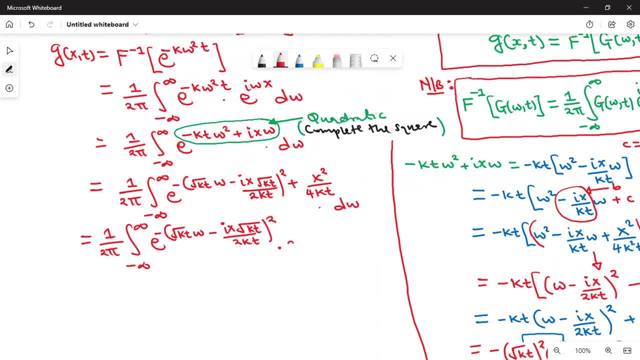 This is squared times another. Another exponential x squared, that should be x. exponential x squared over 4kT, the omega. Now, anything that does not depend on omega can be factored out. Anything which does not depend on omega can be factored out. 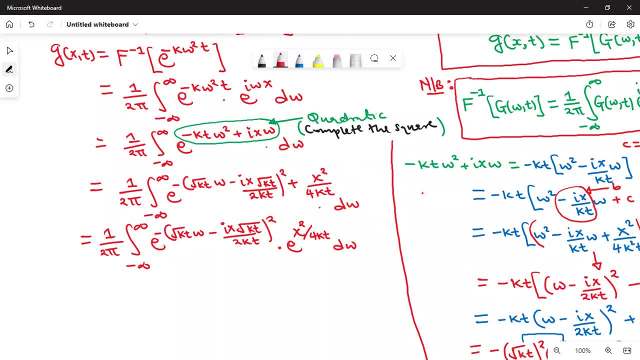 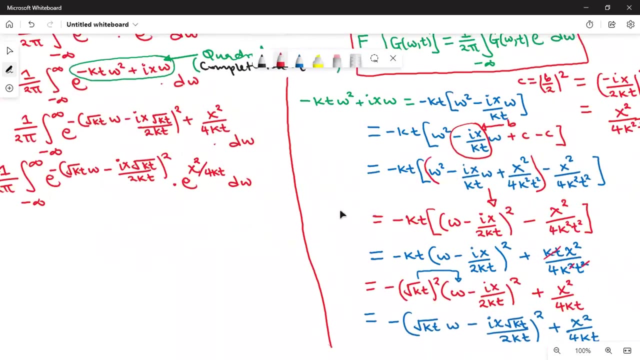 And so what are we going to get when we factor out the exponential x squared over 4kT? Let's see There's some sign that we have missed. Let's just go back to our completing the square. We were adding c and subtracting c. 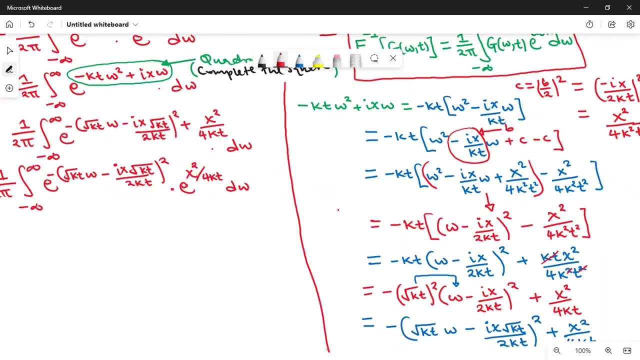 So here It was negative, Then the negative kT will match with that. we have positive kT. And then we missed out something somewhere. Let's just check. Look at the completing square. We added, And what were we adding? 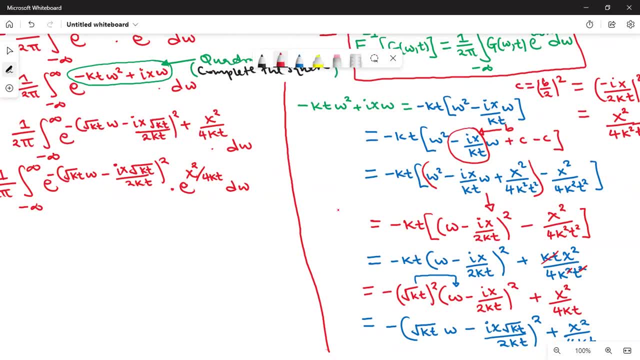 The value of c, We also subtract the same value of c, And so- remember i squared- is negative 1. So we'll expect to have kT, And so that should be a positive instead of a negative. Just a minute. 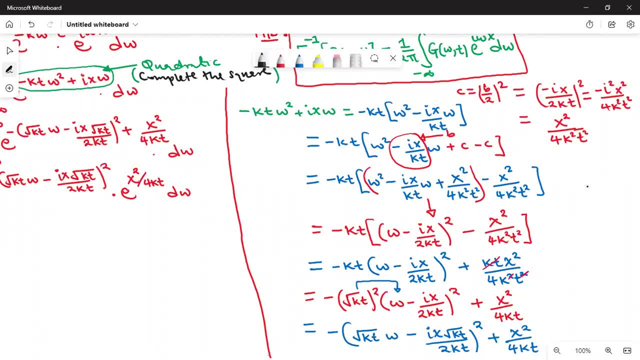 So there's a slight correction here. Look at where we were squaring. It was negative. i squared, Of course, even the negative 1, we did not square This. negative must also be squared. Everything was squared, So that here we need to get negative x squared. 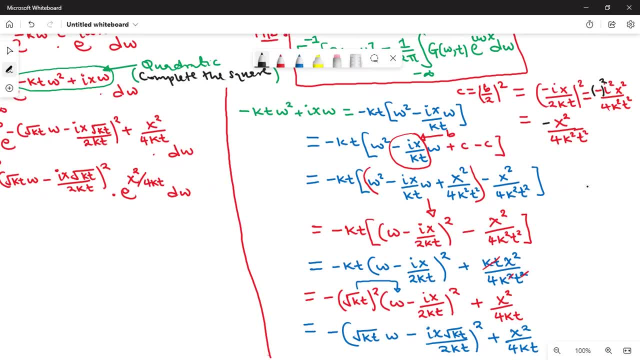 So just change it: Negative of x, squared, That's our c. Our c that we are adding should be negative. So even the sign here must change. We are adding the negative, not the positive. So these signs must change. 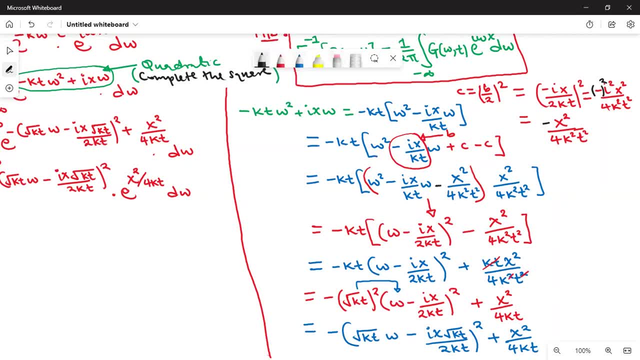 This is we are adding c, Then subtract negative, Negative becomes positive, Then I expect here to be positive, So that again here it will now be negative, Because now you are taking the negative kT Inside. So this should be negative. 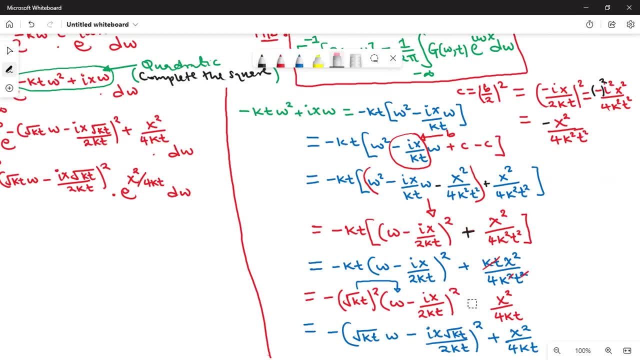 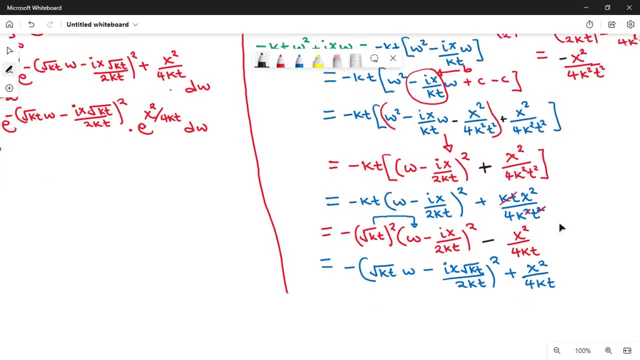 Just a change of sign. A change of sign. This should be negative. Even here it's supposed to be negative. We are just tracking the sign that we left, So even here it's supposed to be negative. And also here it's negative. 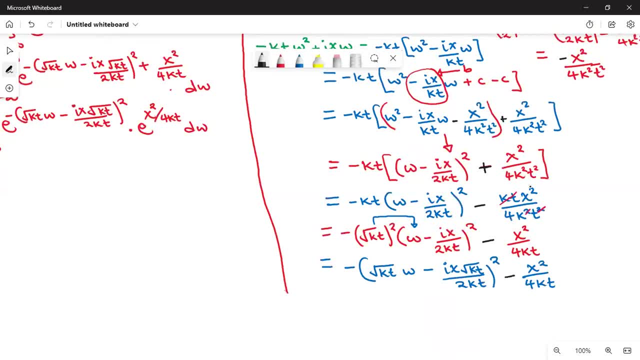 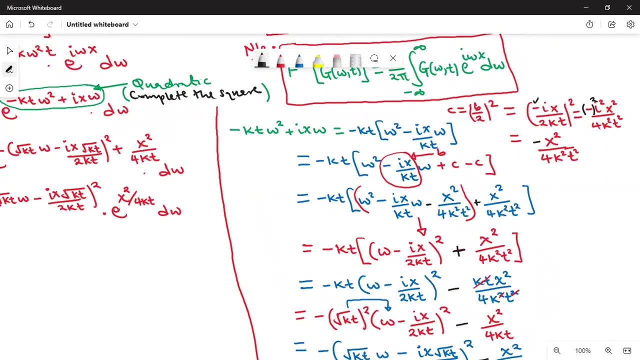 So that correction is negative. So that correction is positive, right, or very important. where did it start from? because you see, here we were squaring: a negative squared becomes positive- it is this one that confused us. and also the i squared is negative. so that's why we still have the negative because of the i squared, but negative one squared. 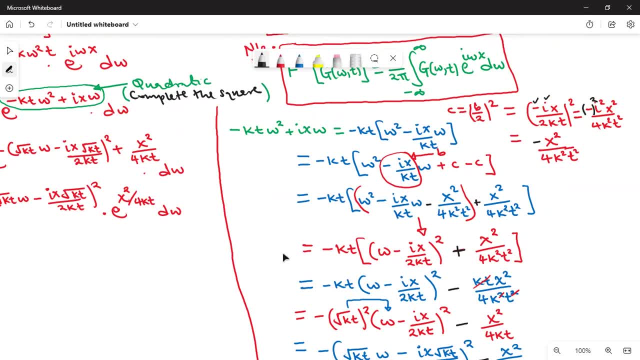 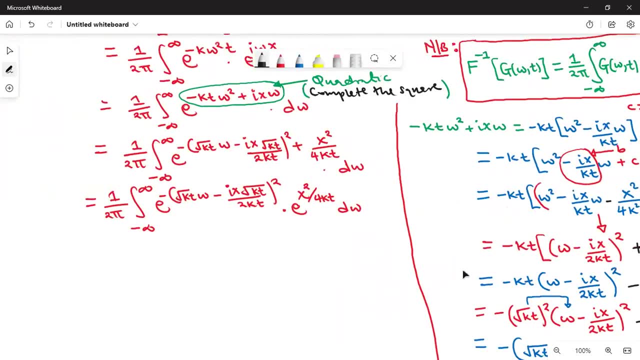 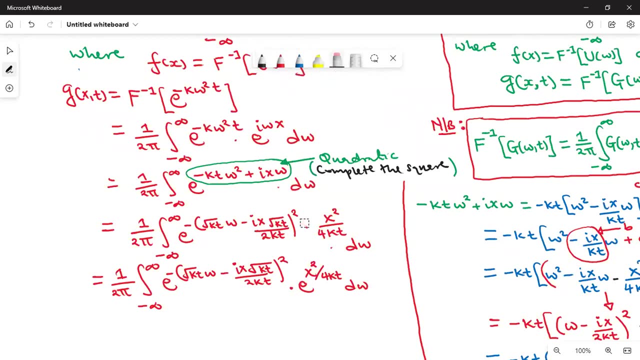 is positive, so take note of that. and so now we have completed the square, let's come back to our problem. we're just tracking the signs here. we expect this to be negative and also a negative here, so this should be minus and another minus here. so that's, that's now okay. 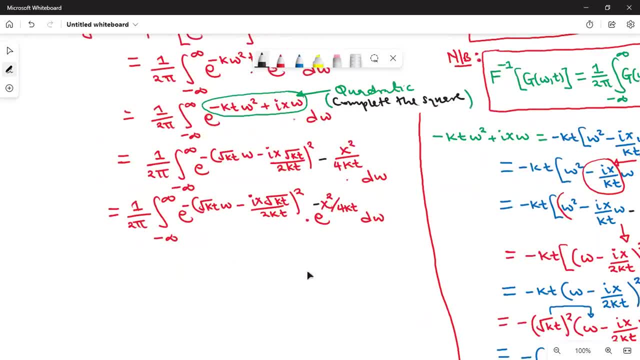 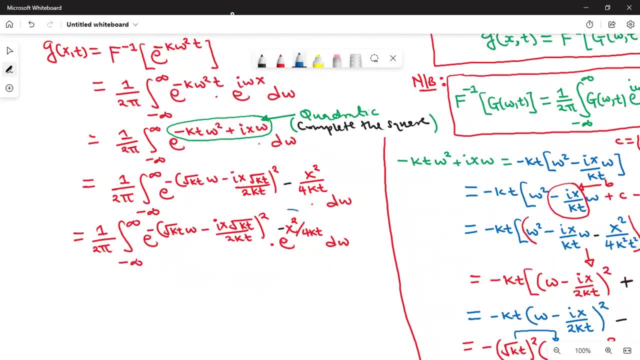 we have corrected it now. i told you that anything that does not depend on x, on omega i mean, you factor it out. so you see this exponential, you see this exponential, you see this exponential. i can't see an omega inside here, so we can as well factor out this. let's take it. 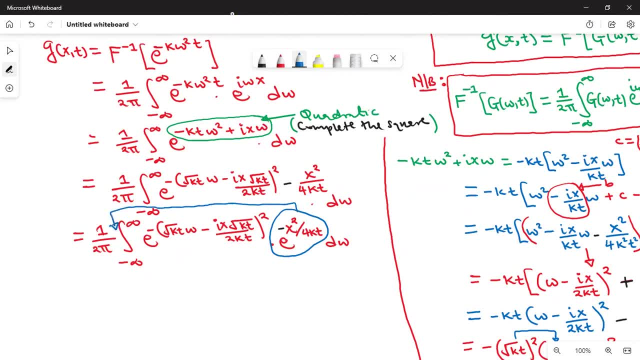 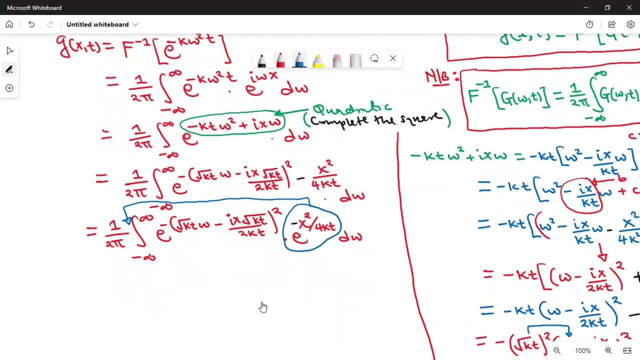 here, so that this integral can now be written as one over two, omega two pi, i mean correction: one over two pi times exponential negative x squared over four k, t. now the integral from negative infinity to positive infinity, exponential negative, the square root of kt, omega minus ix. 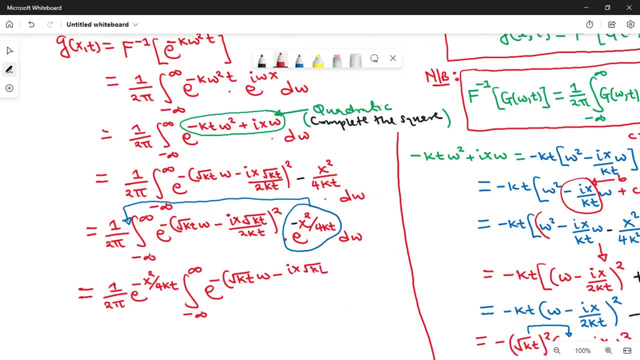 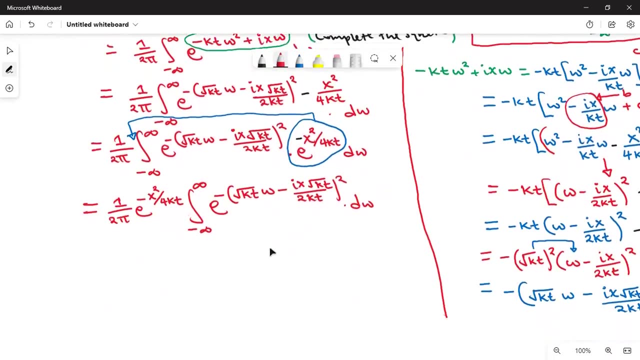 root kt over four, ktк over 2KT, And this is supposed to be squared the omega. Now we are going to use a substitution. I cannot use U, because already we have U as our dependent variable. Let me use Z. 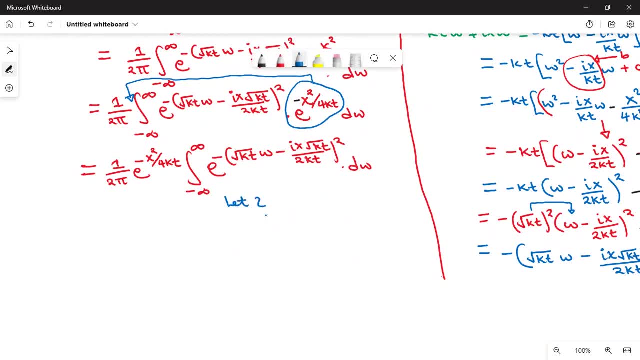 Let Z be equal to the whole of this in bracket. That is root KT times omega minus iota. X root KT divided by 2KT. Let that be Z. So from here you can just say therefore, DZ, D, omega, Because we are moving now from omega to Z. 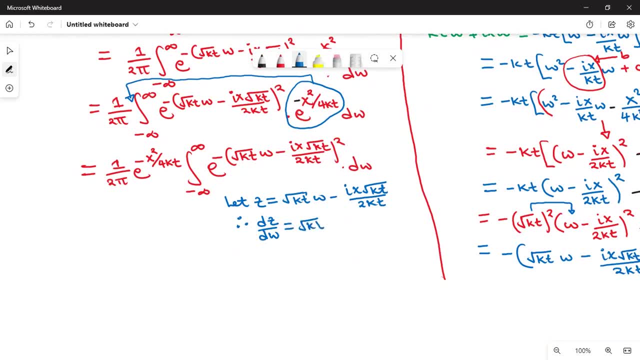 that is simply the square root of KT. You can as well say that D omega when you make it the subject, it will be equal to DZ over the square root of KT. So back to our integral. This integral can now be written as: 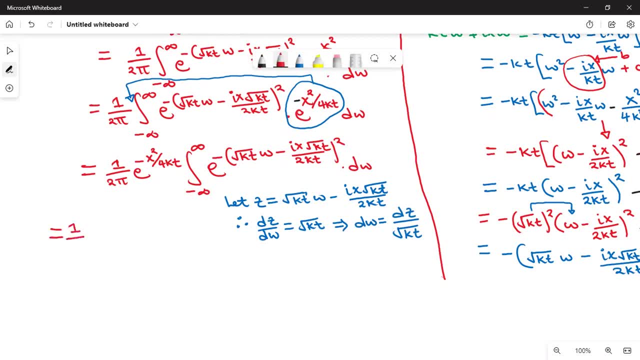 1 over 2 pi. exponential negative X squared over 4KT times the integral. What about the limits? Limits When Z? these are omega limits for omega. Now, what are the new limits for Z When omega is negative infinity? 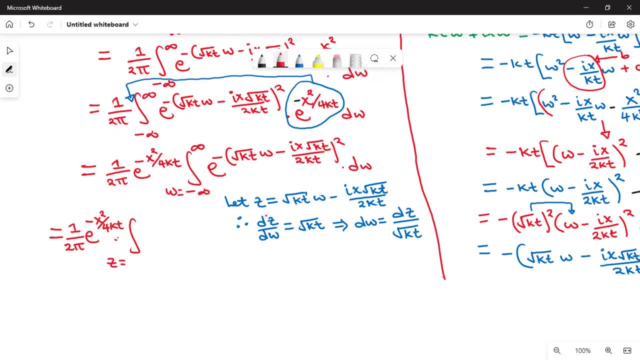 what will be Z? It will also be negative infinity. And when omega? when omega is negative infinity, when omega is positive infinity. here you will find Z is equal to positive infinity. So this will be exponential negative Z. squared times DZ over root KT. 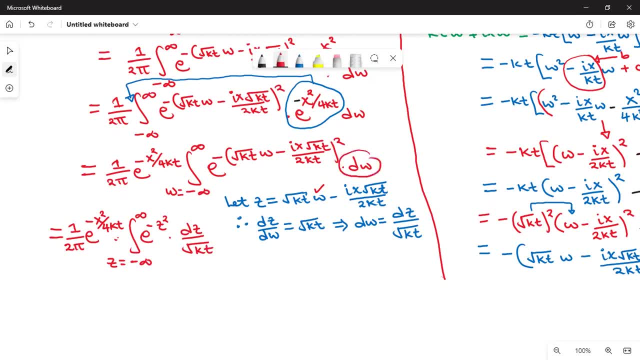 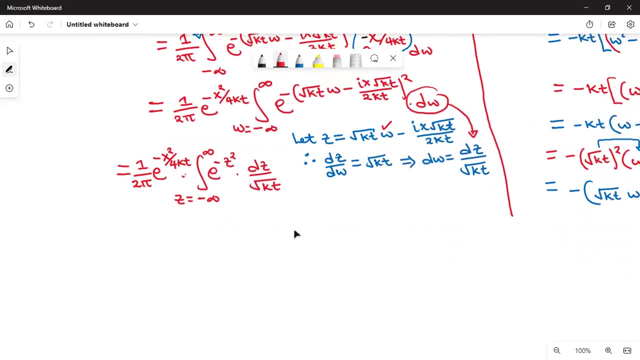 That is D omega. D omega is the same as DZ over root KT. The square root of KT is the square root of KT. The square root of KT is independent of Z, And so we can factor that out so that this can as well be written as: 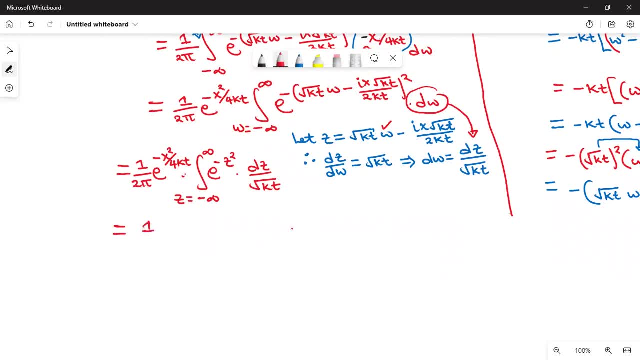 1 over 2 pi times. I can see this: the square root of KT times the square root of KT times the exponential. exponential negative X squared over 4KT, Then the integral from Z is equal to negative infinity to positive infinity. exponential negative Z squared DZ. 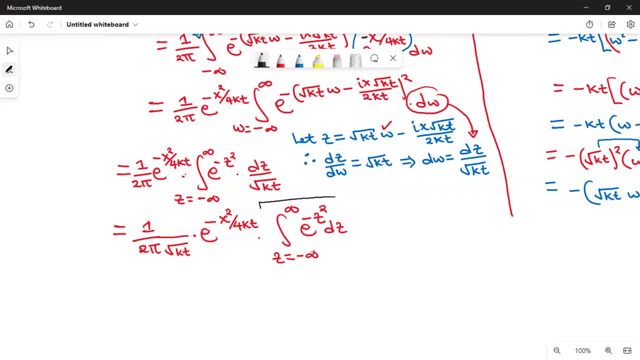 Now from the properties of error function or from the gamma and DZ and the beta functions. the square root of exponential negative Z squared DZ from negative infinity to positive infinity is always equal to the square root of pi. I said the integral of exponential negative Z squared DZ. 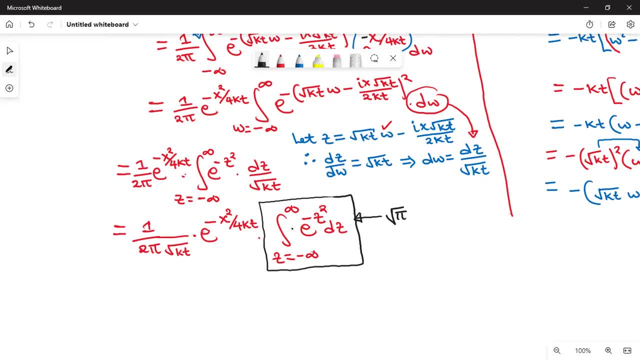 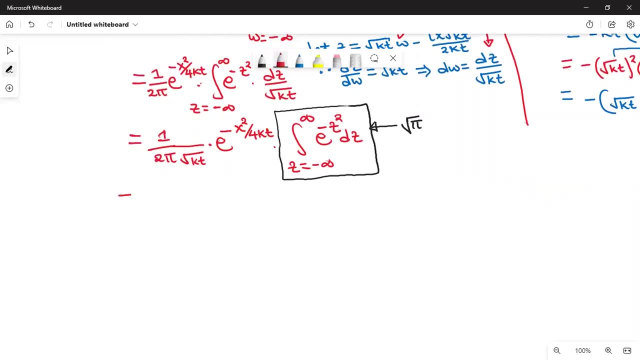 from negative infinity to positive infinity should give us root pi. So therefore this can now be written as the square root of pi over 2 pi times the square root of KT times exponential negative X squared over 4KT. And you see, I can see there's pi in the numerator. 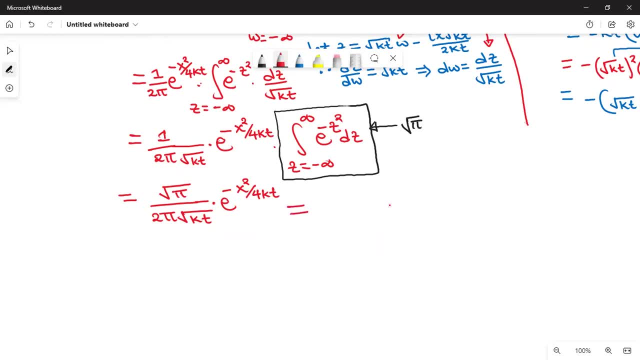 another pi in the denominator, I can combine them. Look at: we have pi raised to 1 over 2 divided by pi. So it's the same as. this is the same as pi raised to negative 1 over 2, which is the same as 1 over root pi. 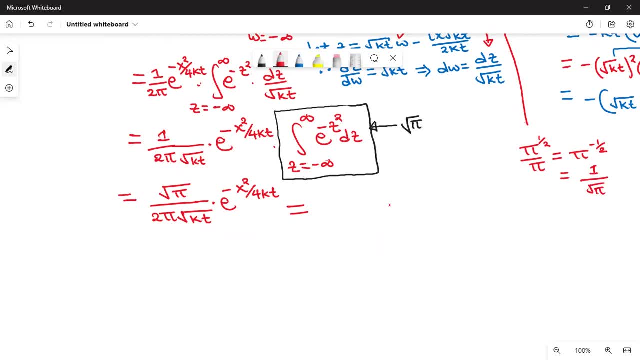 That's what we have, So that this can now be written as 1 over 2, the square root of now, even this root pi and also this root KT. So I've just combined them under one square root, So that would be pi times KT. 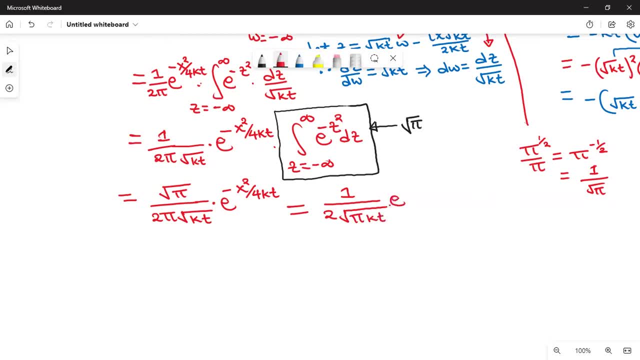 exponential negative X squared over 4KT. So that's what we have Now. this is our. you can just say, therefore, G of X, T. G of X is equals to this, So hence we need to find G of X minus S, T. 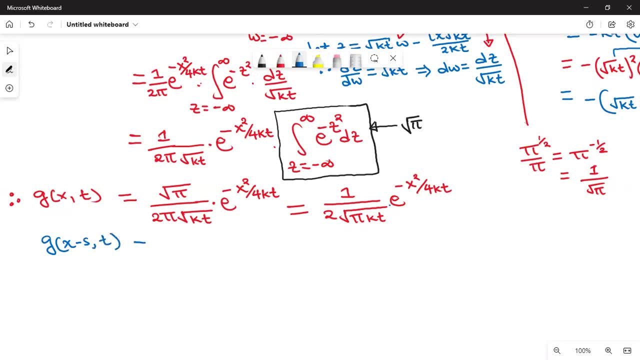 So where there is X, you put X minus S. So what will this be? It will be 1 over 2, the square root of pi KT exponential negative. Now we are replacing X by X minus S, So this will be X minus S squared. 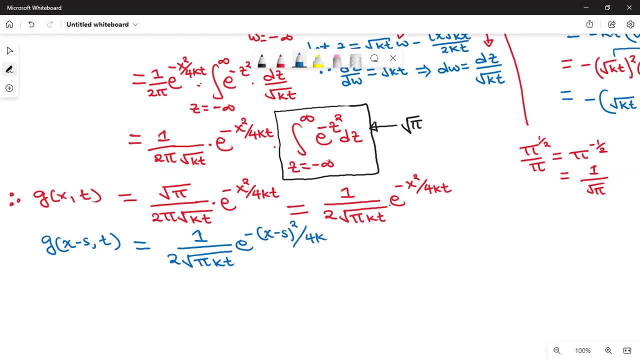 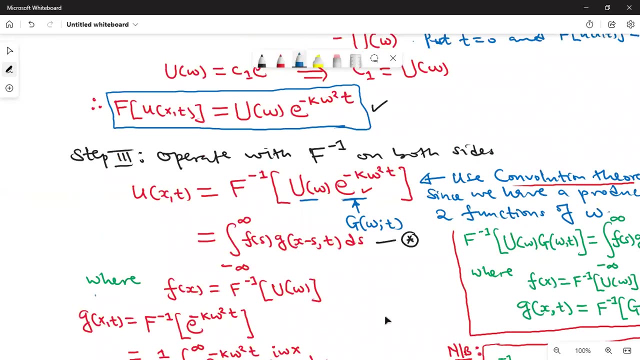 over 4KT. That's what we have, And now our particular solution. we now replace what you have found. Look at where we started. All of this was just to find G of X, T, As I have explained, I was very slow. 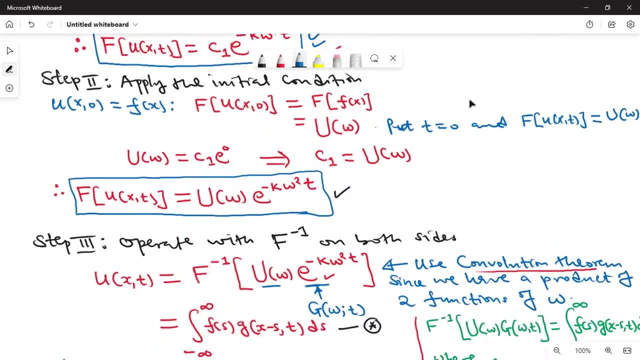 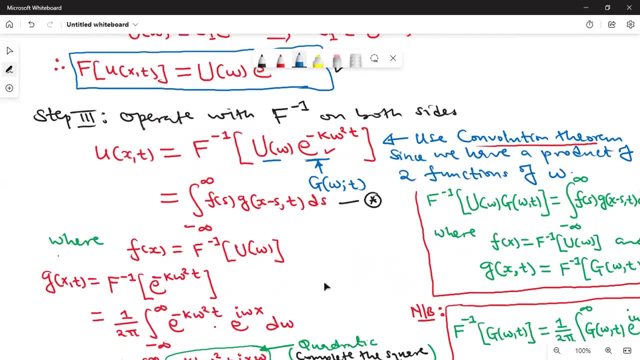 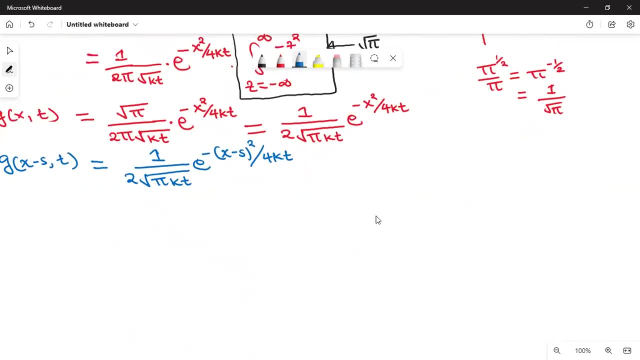 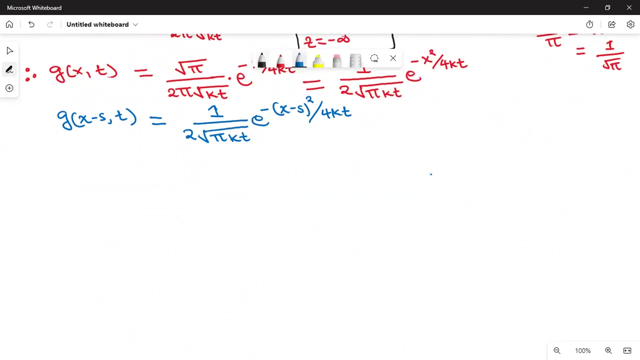 so that we understand each and every concept. So we'll come back here to our equation star. So what will be equation star? How will it look like? That will be our particular solution. So, therefore, our equation star will now become equation star. 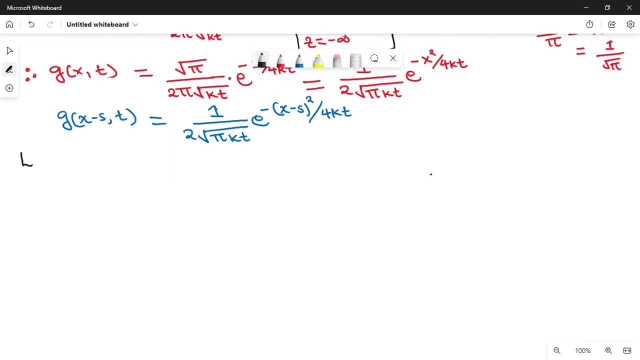 Now we are going to substitute this into equation star, So let me just write here: equation, equation star. Look at our equation. On the left we had U of X, T. What about the right-hand side? It is the integral from negative infinity. 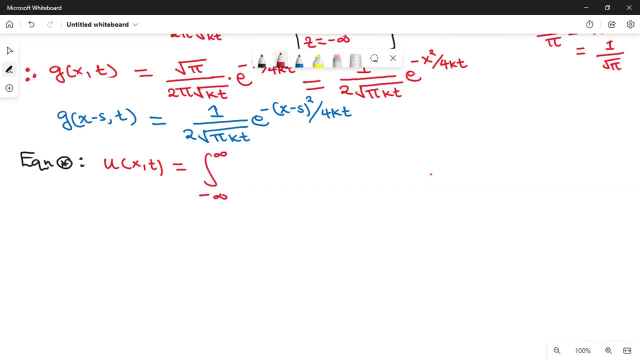 to positive infinity of F of S. F was arbitrary, so I don't know F of S because it's an arbitrary function. Then times this other one, G of X minus S, times T, So times one over one over two. 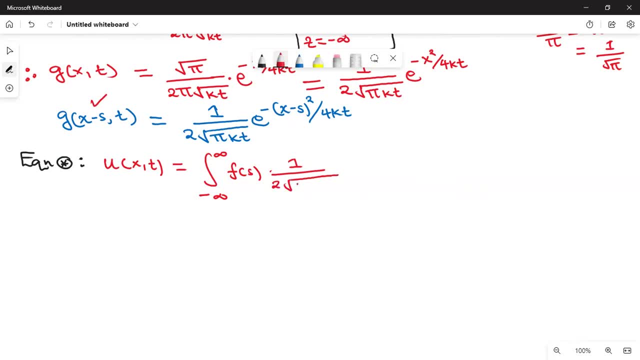 root pi K T. So root pi K T times exponential negative X minus S. This is supposed to be squared everything over. for K T, That's X minus T, And right here Y on the right. So do you remember this? 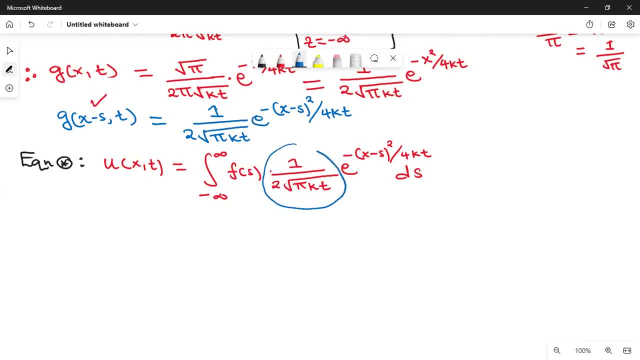 We have to take anything that does not lie on the right side. And what should we do? We take, what should we add this time? So the final tangent is now equal to power over y, the first equal to 1 over. 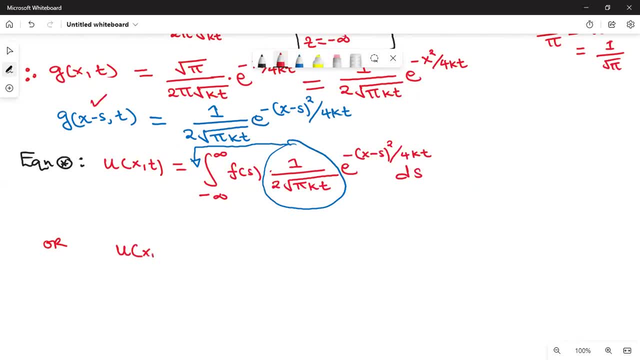 K T by K T. So this here: this means that we update state function Chapter one: one over two root, one over two root, pi kt. that's outside then the integral from negative infinity to positive infinity, f of s times exponential negative x minus s. 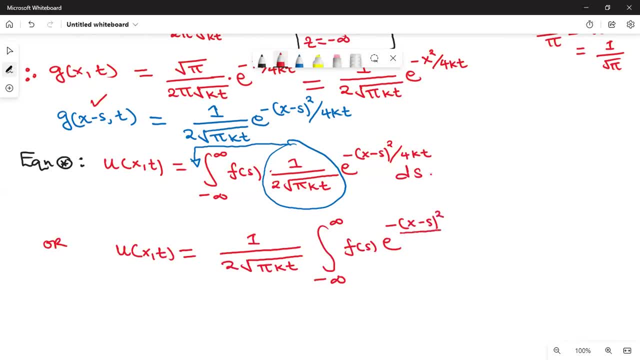 is supposed to be squared everything over for kt ds. this is our solution. if you knew the function f of s, then you can be able to find the particular solution corresponding to that given function. but in this case we are not given the function f of f of s, so we leave our solution.